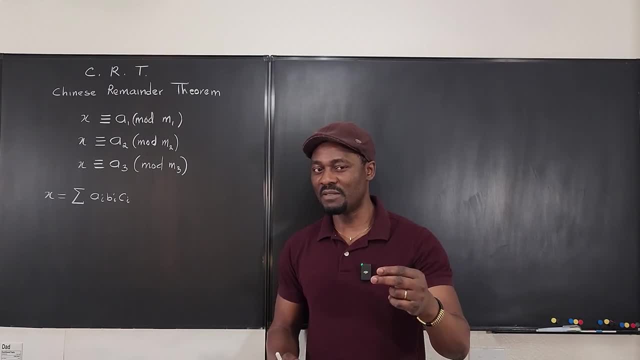 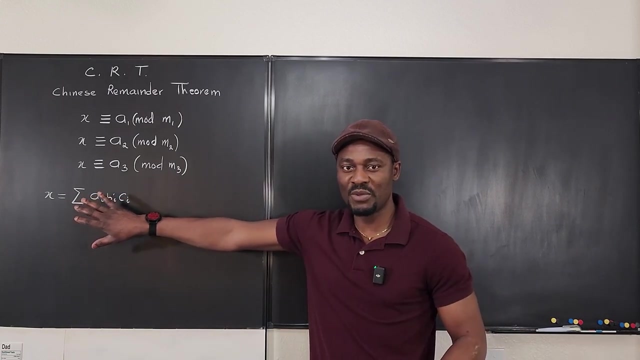 And then, if I take the same number and divide it by seven, the remainder is going to be three. Okay, The confusion is beginning to set in because your guesses are becoming more and more inaccurate. So the Chinese remainder theorem will help you figure out. 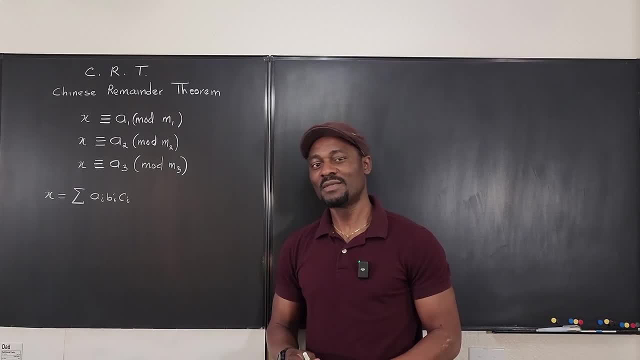 what particular number is divisible by three. And then I tell you: but if I take the same number and divide it by five, the remainder is going to be one. So that simply means particular number I'm referring to. Let's get into it. 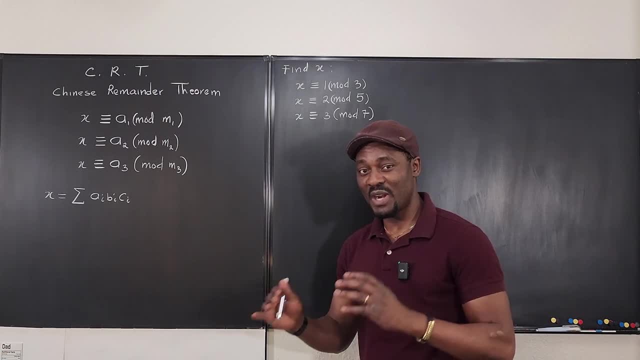 Let's get into it. Let's get into it. The example problem that I gave when I started can be written this way: When x is divided by three, the remainder is one. So we say x is one mod three, That is, x leaves a remainder of one. 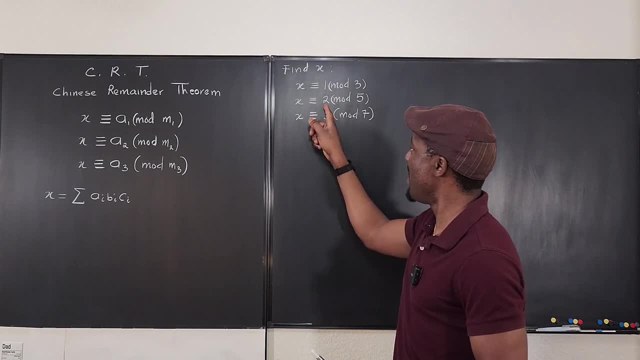 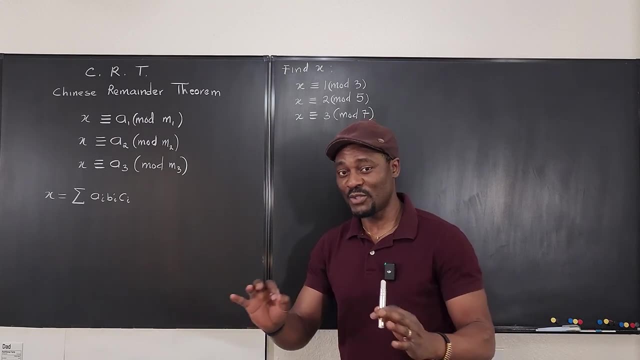 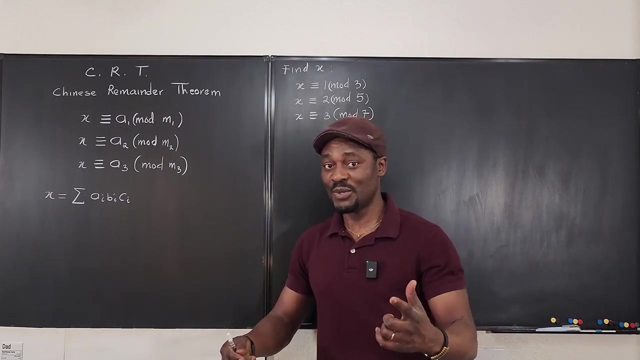 when divided by three. When divided by three, the same number that I give when I started, from 1 to 1.. same thing: x leaves a remainder of 2 when divided by 5, and that's the essence of the whole modular expressions that we have. so, as you can see, 31, for example, will be 1 mod 10, because when 31 is, 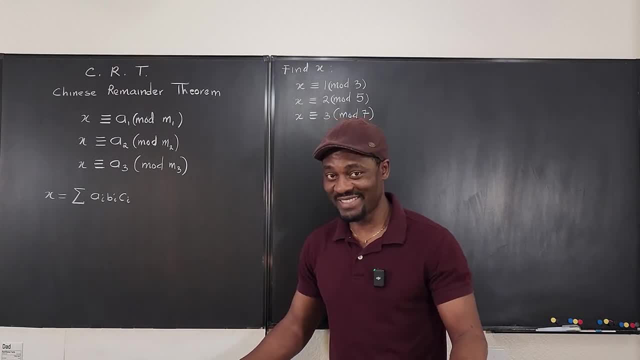 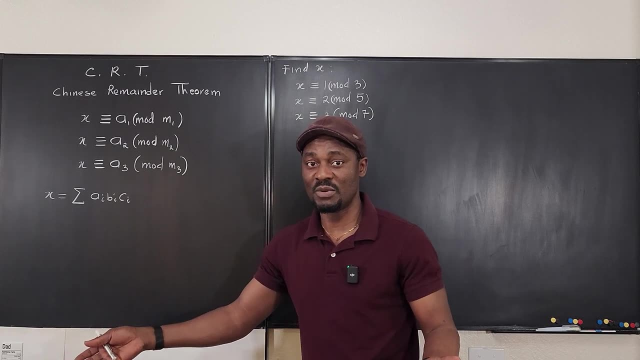 divided by 10 and the remainder is 1, right, okay, that's how, why we write it. we write: okay, 31 will be 3 times 10 plus 1, where the 1 is the remainder. so that's the whole concept here. so why is it? 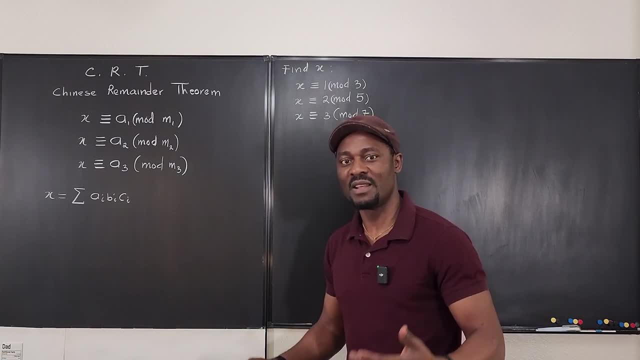 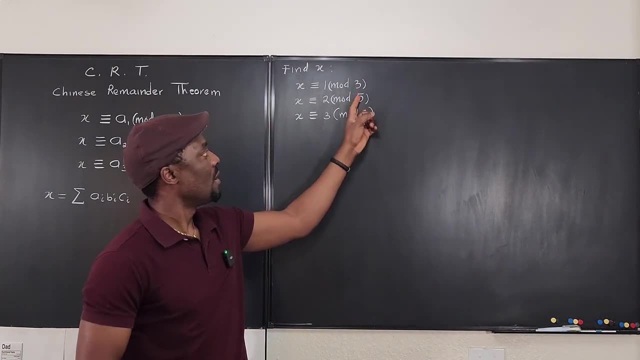 called the chinese remainder theorem. obviously it was invited, invented by the chinese. so how does it work? you see, the numbers i have chosen here are all relatively prime. that is, no number shares a common factor. there's no number that divides three, that divides five, that divides seven. 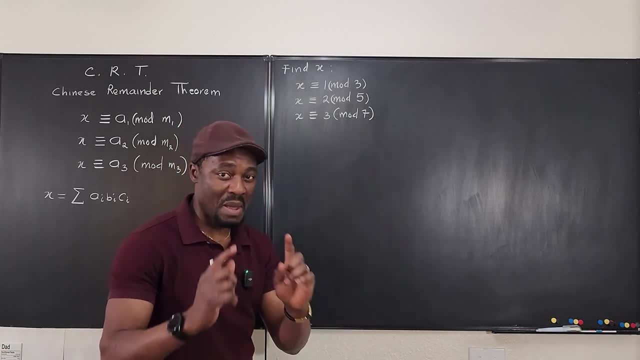 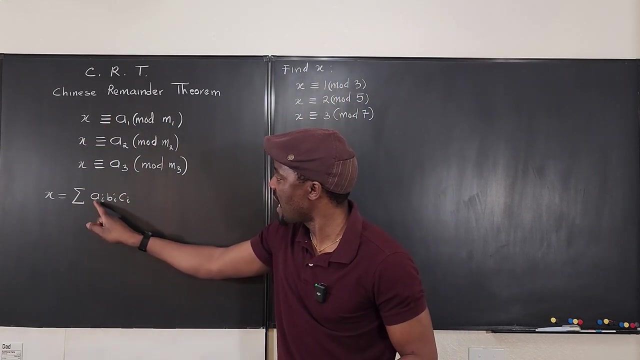 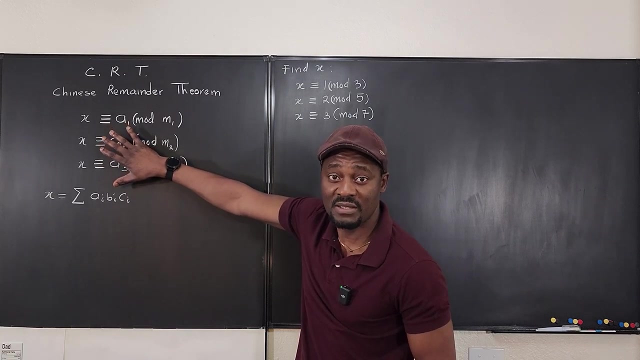 no, everything is. they're all relatively prime, so remember that's a precondition for the chinese remainder theorem to work: the numbers cannot have common factors. okay, so now let's go. i already labeled this, so forget about this question. let's focus on this and see what a is, what b is and what c is, because there are three different divisions that i've expressed. 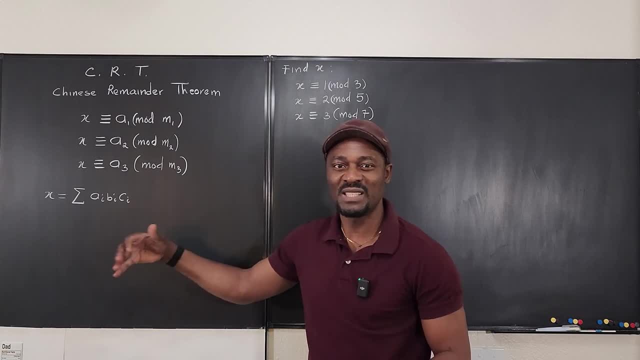 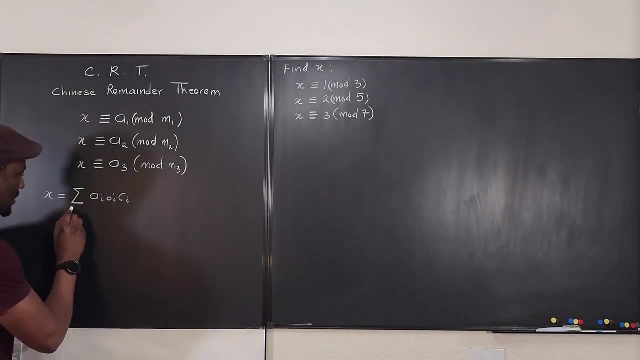 you're going to have three of these, so the sum of these three abc's becomes your answer. so because i have three here, i'm going to. so this is from i to n. so here, since n, since n equals 3, my answer is x equals a1, b1, c1 plus a2, b2, c2 plus a3, b3, c3 and, as you can see, 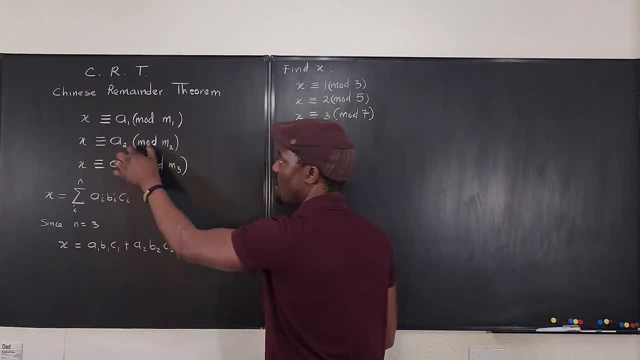 this one is attached to the first one, the second one and this is the third one. so what is a1, what is a2 and what is a3? let's i'm just going to work through this so you can see that the first one is a2 and what is a3, so you can see all the ingredients that we need in making this. 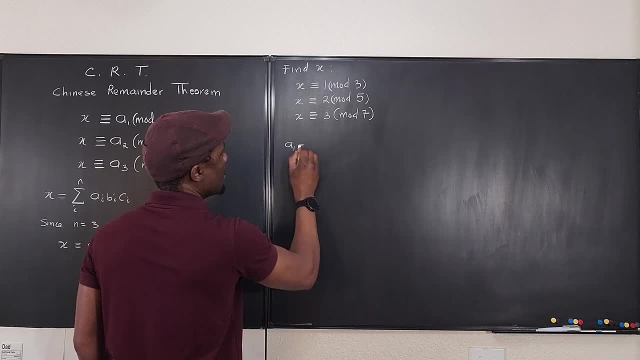 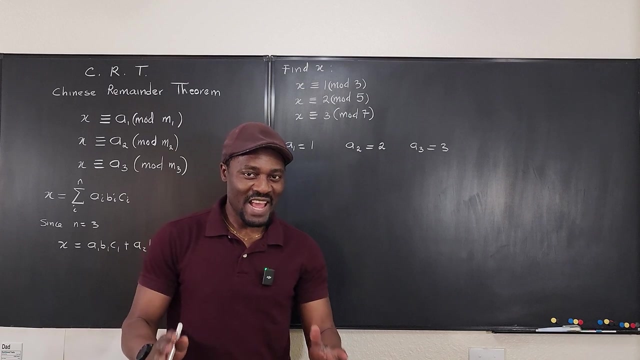 calculation come alive. i'm going to say: a1 is equal to the first number here. so this is the first problem. my a1 is one. what's my a2? is this number two? okay, oh, let's write it this way. so now the next thing i need you to write is your c, because c is easy. you don't need to do any. 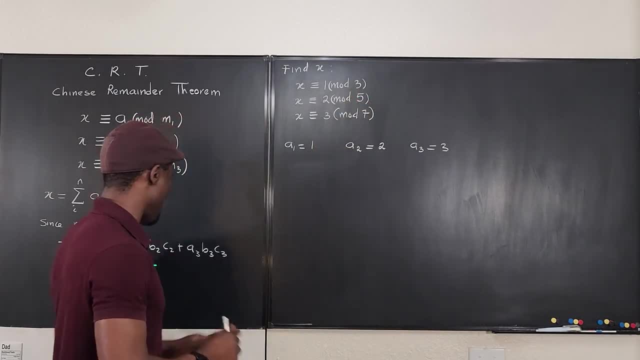 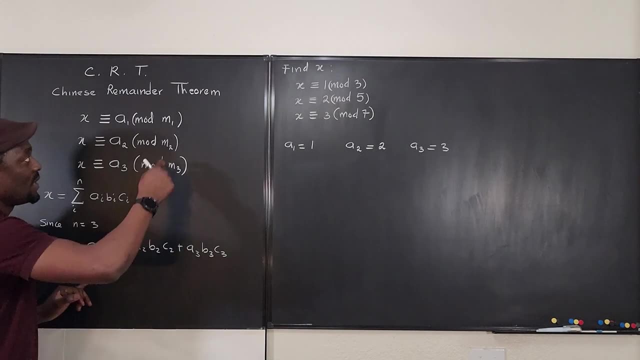 calculation, because these numbers are relatively prime. what will you do? you're going to write a1, that's a4 here, and of course, b2, c, two, 1 and a3, c2. and now, if you do something in the order here, let's say this is c. you did write c 1, that's a 9, um, that's a n, and there you go, three plus 3. 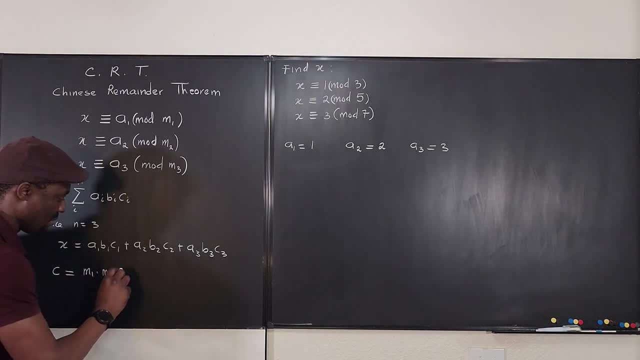 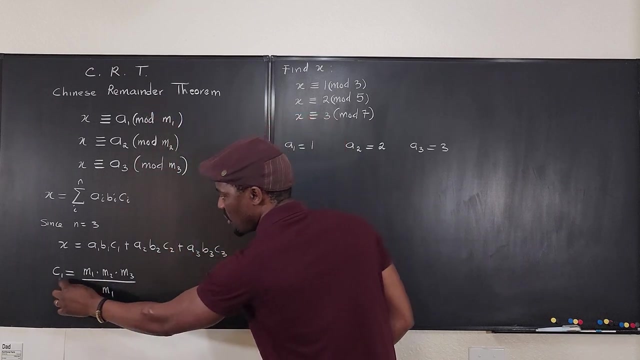 which equals 9? how many numbers did it want to WIN? what was c 1? yeah, quite a little too small and i left about 12 of them. that's a only one, it's not a number of 7. math connects A1 with num3 initiative, so Ce n. 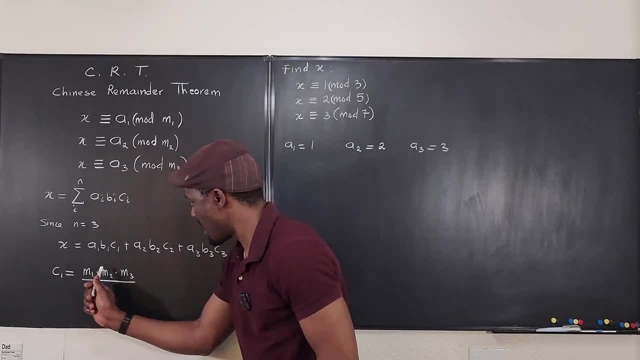 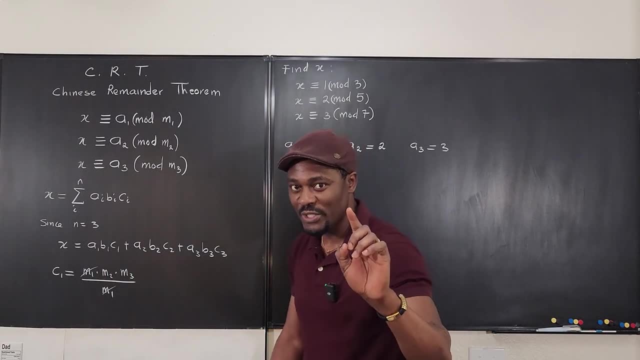 It is these multiplied together, divided by m1, and, as you can see, this cancels this out. So what's left is just the product of the other two numbers. So in order to get your c's in this formula, you just need to multiply the other two numbers together. 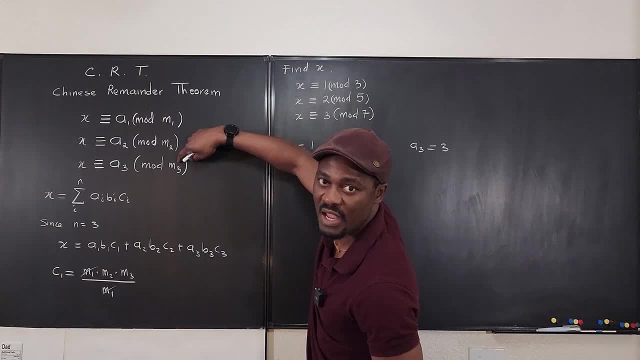 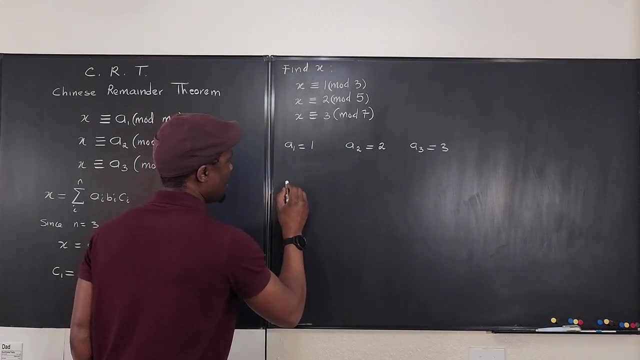 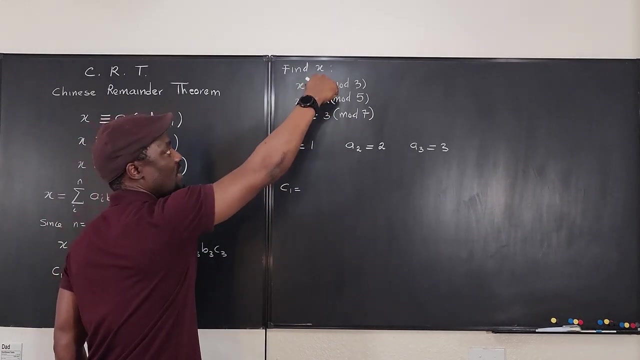 So my c1 will be m2 times m3.. So let's write it here, Let's put a formula here and say that my c1 will be equal to m2 times m3.. So I'm dealing with this first one. 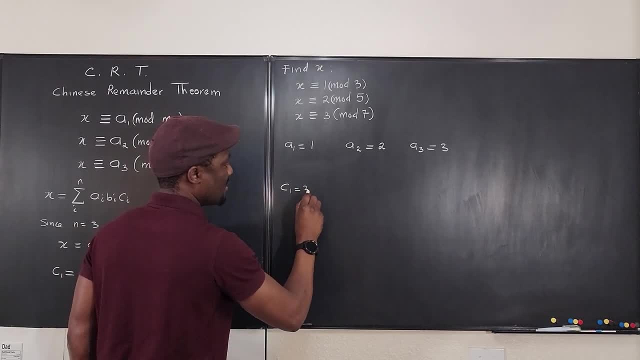 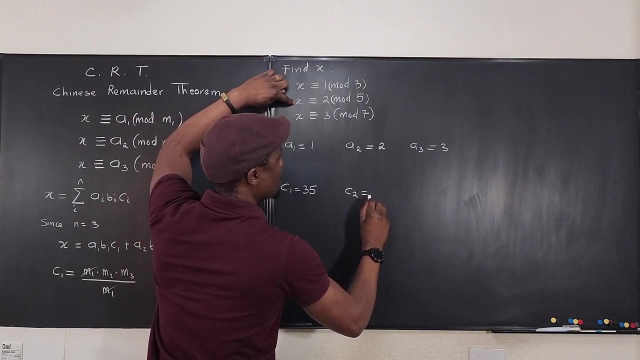 It's going to be the product of these two, which is 35. Okay, so write that down if you're taking notes. Okay, the second one will be my c2.. So you're going to skip this, and then you multiply 3 by 7, which is going to be c2 is equal to. 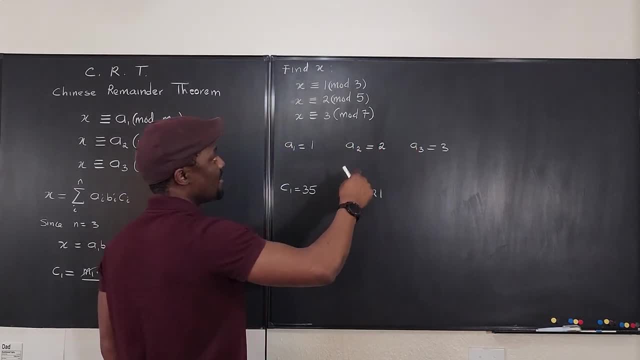 21. And what is c3?? c3 is going to be: we skip this, we multiply this, it's going to be 15.. c3 equals 15.. So we've gotten six of the nine things that we need. 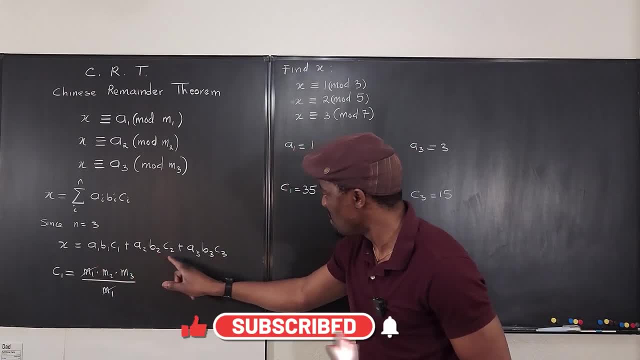 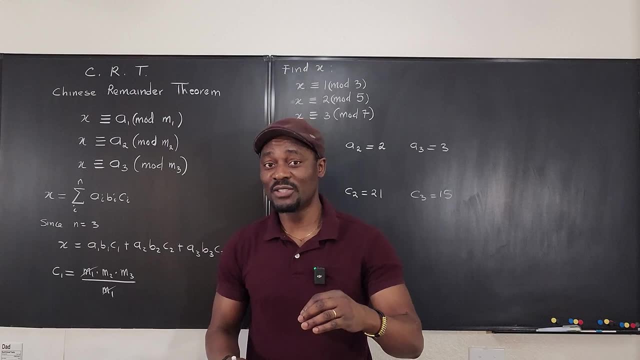 Remember, we need nine, So we need to go get all the b's. Now, what are the b's? This is where it gets interesting And this is the only part where your number, your knowledge of number theory might be required, will be required. 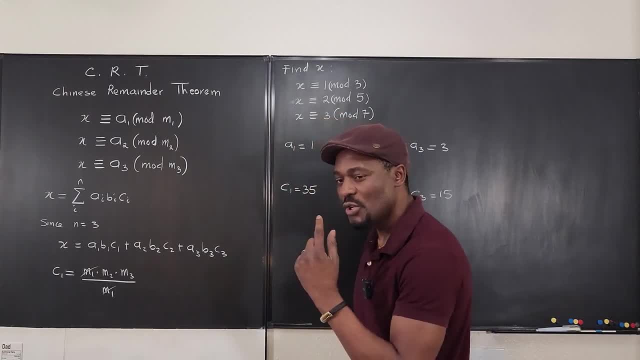 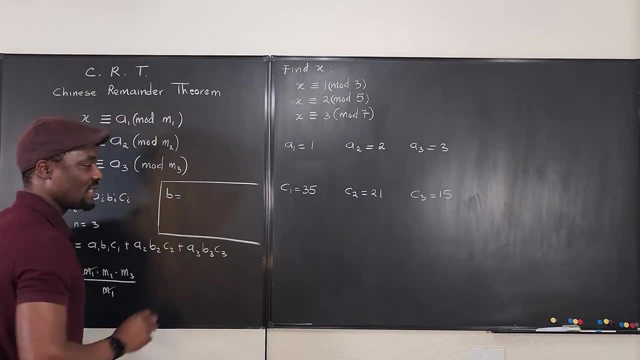 But I'll make it. I'll make it as simple as possible. So how do you get your b's? By definition, let's put it here, The b is always equal, The inverse of c. See, each of these c's are these numbers. 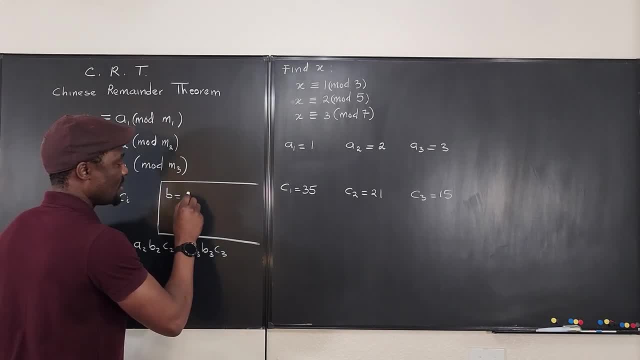 So you're going to write what the inverse of c will be. So b equals c inverse mod m1.. Okay, Now it's not complicated. I'm going to take an example, I'm going to do it here and then erase it. 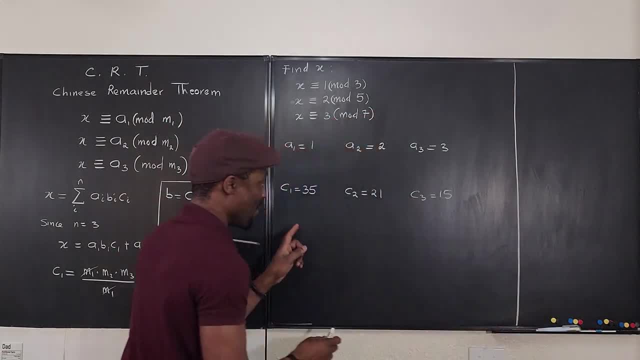 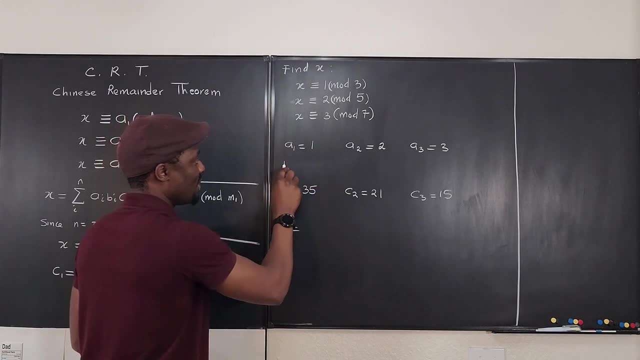 Or let's do it on the side, Because now we can write our final answer. Remember, our final answer is going to be equal to a1 times b1.. Well, we're going to write b1 here. We don't have it yet, but we're going to write it. 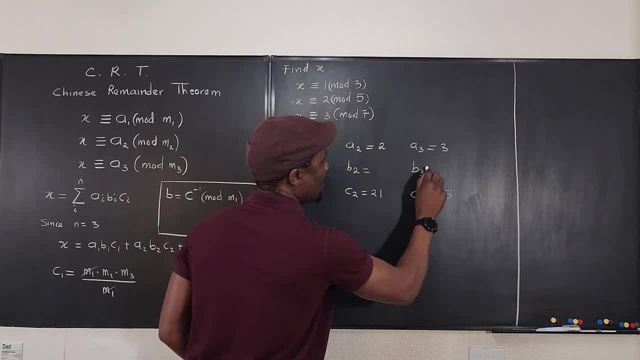 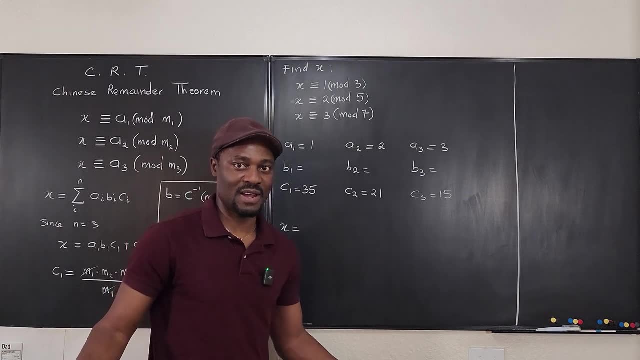 b2.. And then we have b3. So we're just going to multiply this way, multiply this way, multiply this way, add them together, And that's our final answer. It's super easy, Okay. So now? 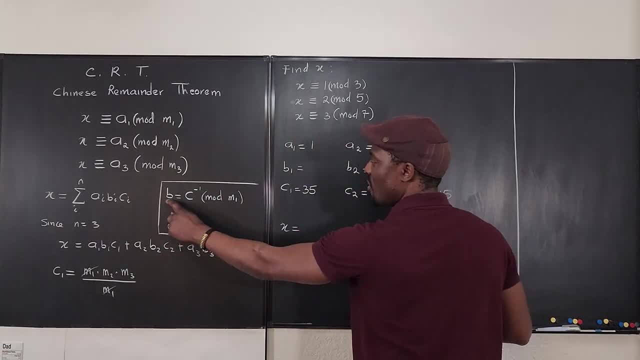 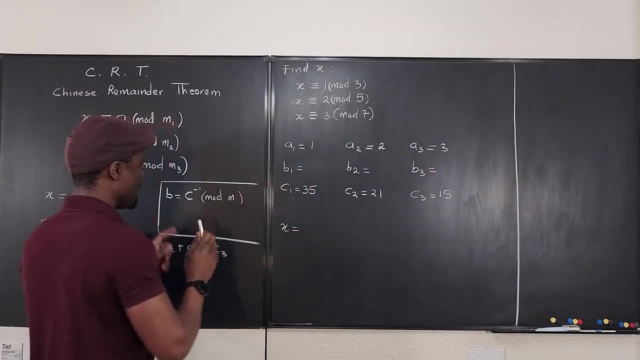 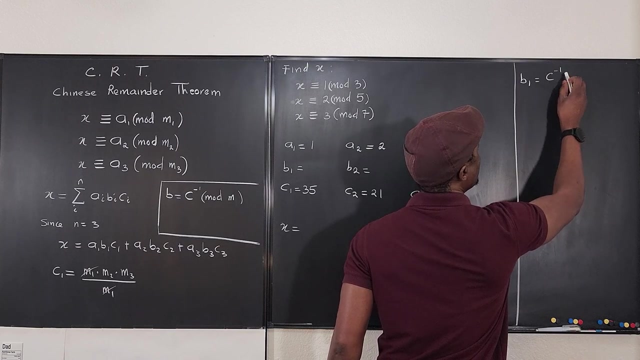 But how do we get b1? Using this formula, your b is the inverse of c mod m1.. That's mod m. Let me do mod m. So if you're dealing with b1, let's write b1.. So b1 is the inverse of c1 mod m1.. 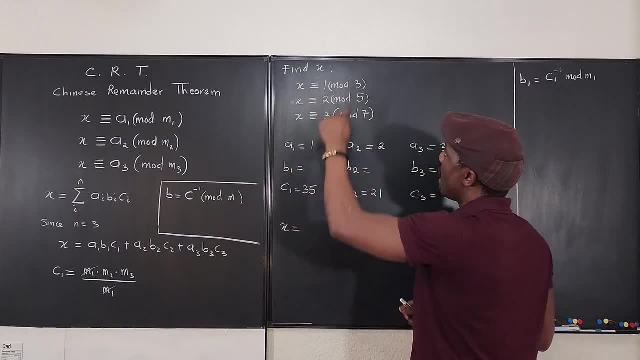 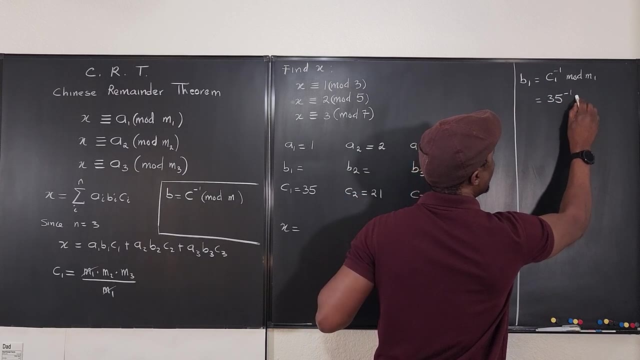 So let's go back. What's our m1?? Right now, our m1 is 3.. Okay, Based on the definitions that we have, m1 is 3.. What is our c1? It's 35. So we're going to say this is equal to the inverse of 35 mod 3.. 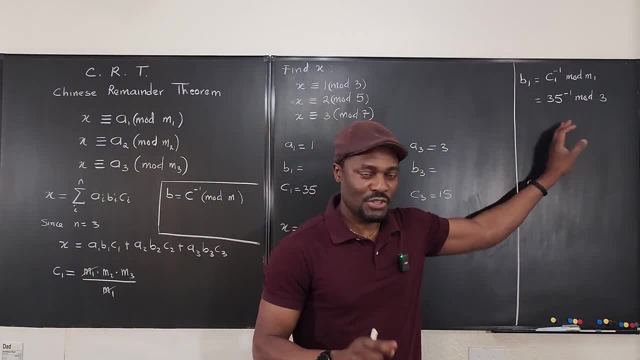 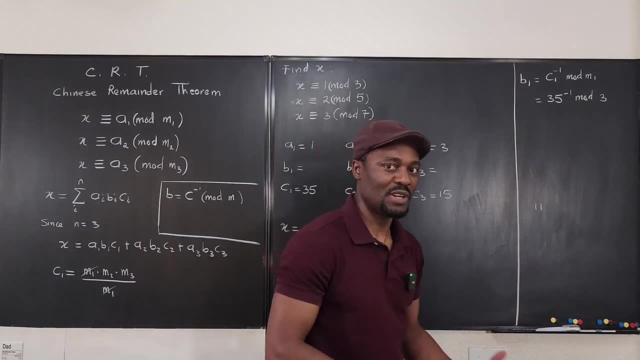 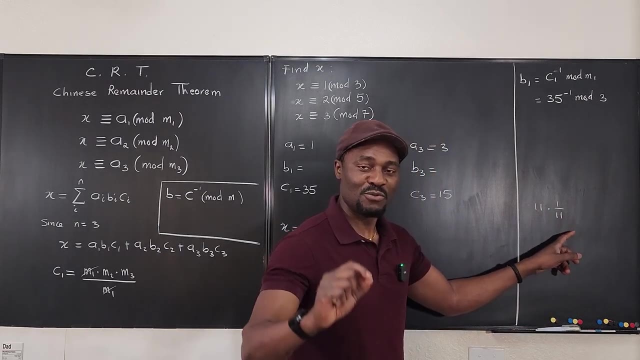 Okay, The inverse of a number. You see, if we're dealing in mod 10, the inverse of 11 is simply 1 over 11.. Because 1 over 11 is the number by which 11 will be multiplied, So that the remainder is 1 when you divide by 10.. 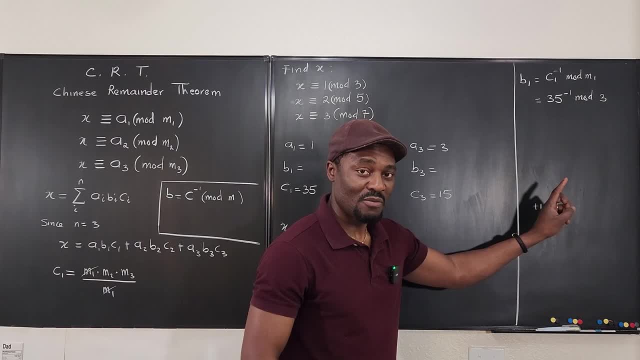 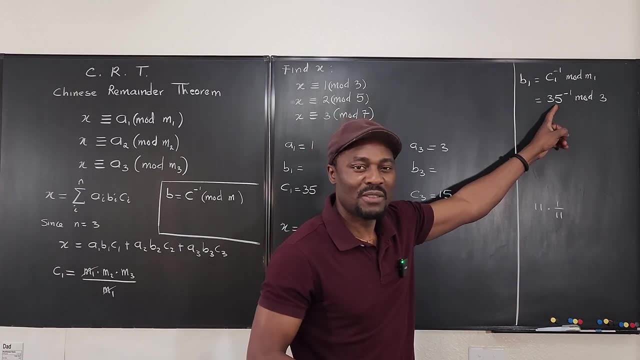 See: 11 times 1 over 11 gives you 1., And if you divide 1 by 10, it's just 0 remainder 1.. So whatever you multiply 35 by to get a remainder of 1, when you divide that answer by 3 is your number. 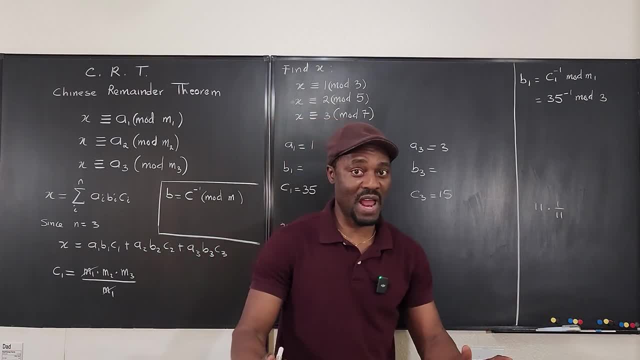 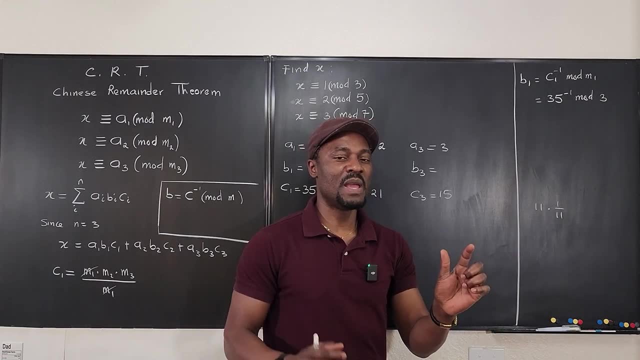 Let's start with 35.. Usually you start with 35.. Remember no fractions. You have to look for another number. So if I divide 35 by 3. It's going to be 11, remainder 2.. So no. 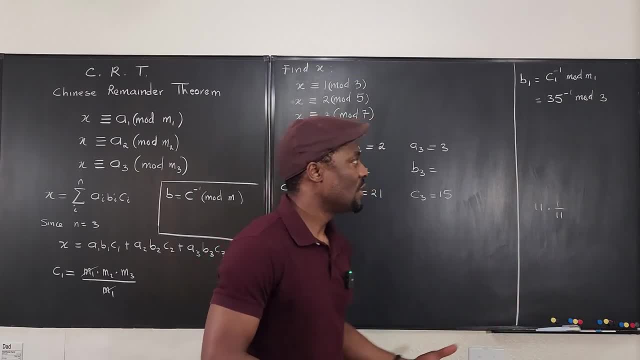 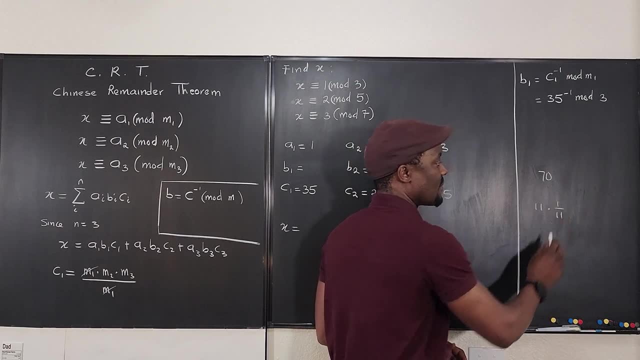 So I'm going to have to look for a number to multiply 35.. So the first number you want to try is 2.. So if you multiply 35 by 2, you're going to get 70.. If you divide 70 by 3, well, it's going to be. 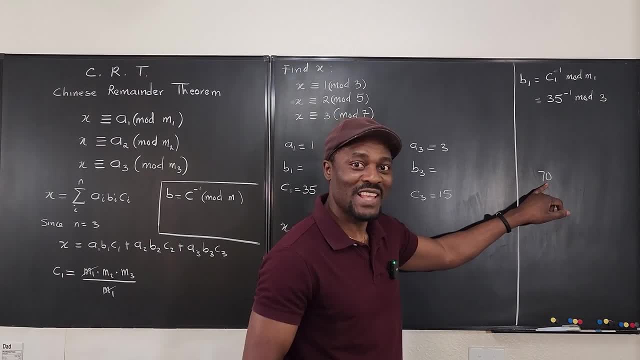 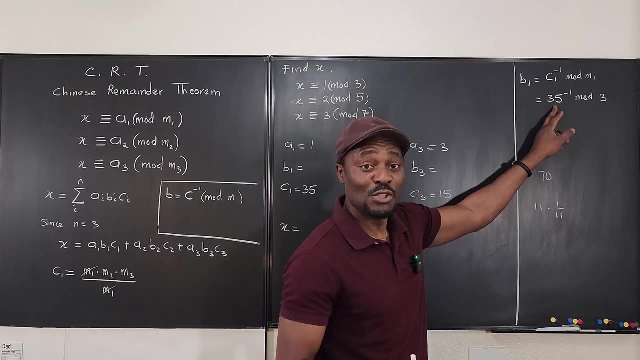 Oh, that's 69 remainder 1.. So you notice that once you multiply 35 by 1, you're going to get By 2, rather Your remainder is going to be 1 when you divide the answer by 3, because you're going to get 70.. 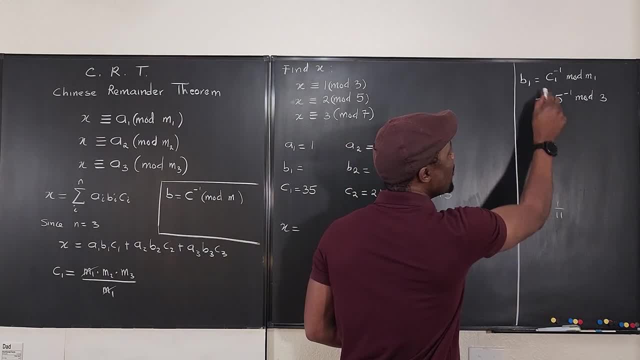 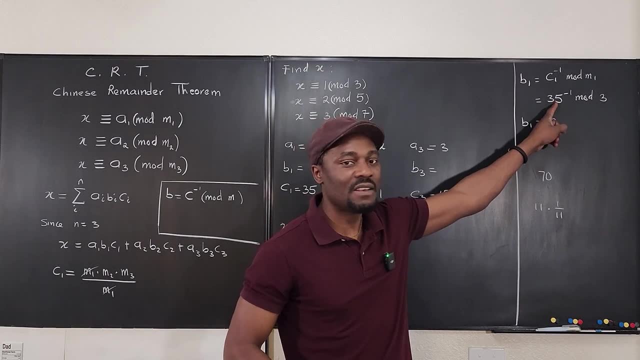 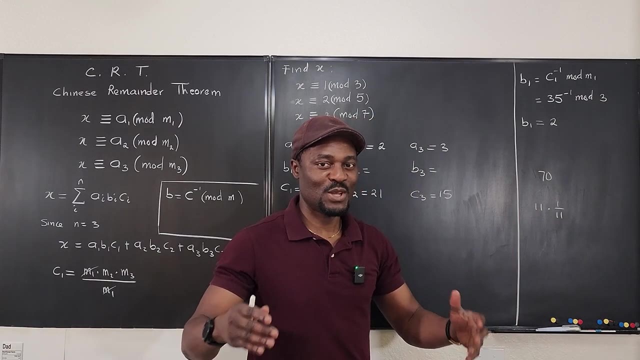 So it simply means that your b1 is equal to 2.. Because 2 is the inverse of 35 when you are in mod 3.. Because 2 is the smallest number that you multiply 35 by to obtain 1 as your remainder. 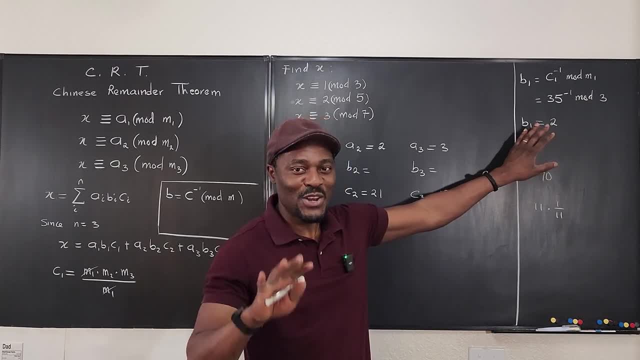 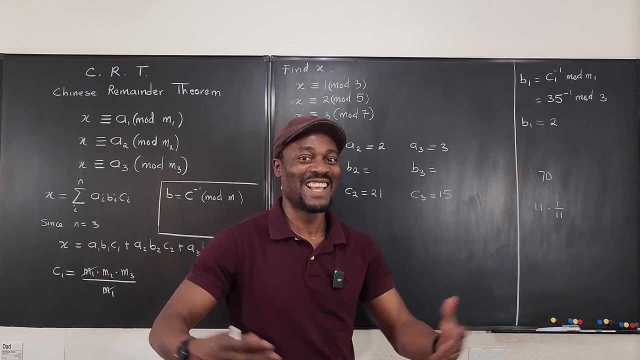 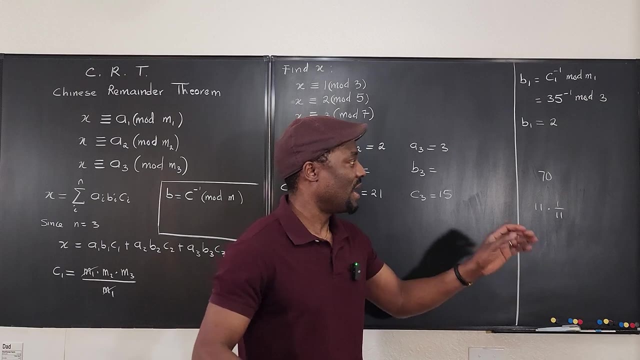 There are other ways to get this, But because I know not many of my YouTube viewers are number theorists- okay, If this was a number theory class, we would use the matrix method or use the division algorithm from Euclidean algorithm, But right now I'm just going to make you just use mental math. okay, to do it. 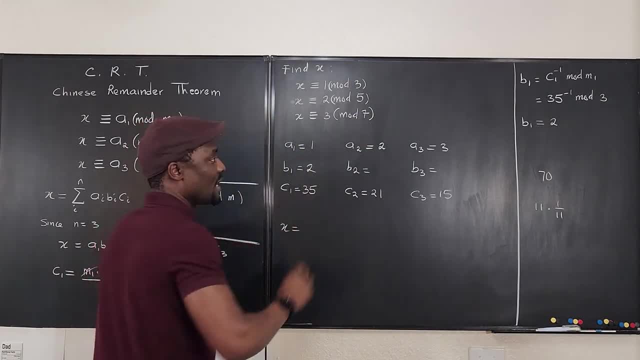 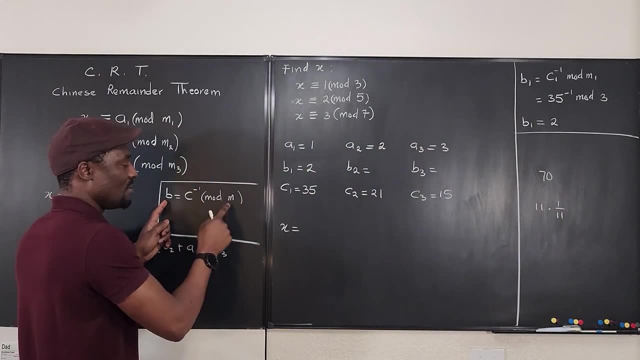 So that's what we have: b1 equals 2.. Now let's try the same thing for b2.. We use the same formula For b2, it's going to be the inverse of c2.. Mod m2.. 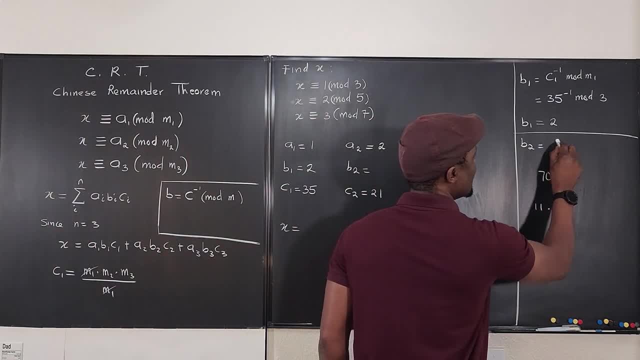 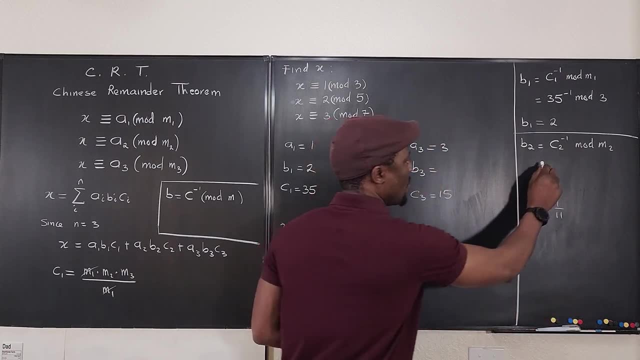 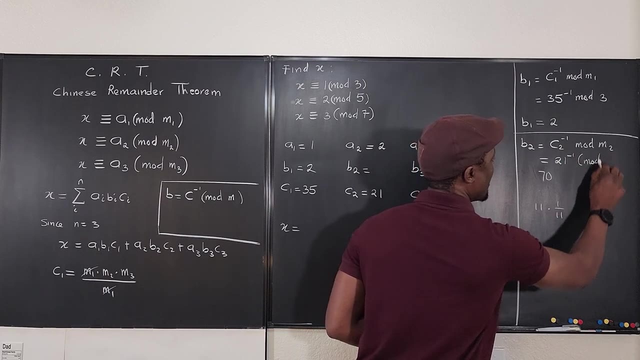 So we're going to say b2 equals the inverse of c2. Mod m2.. But what is What's c2?? We said c2 is 21.. So what's the inverse of 21? Mod What's m2?? 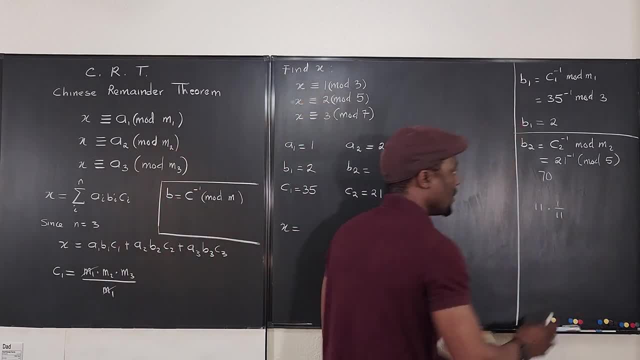 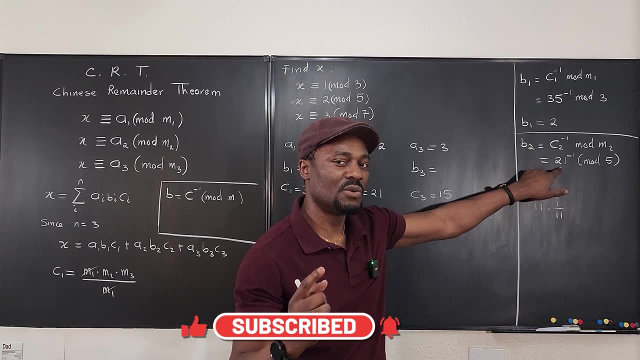 m2 is 5.. So what would you need to multiply 21 by, So that, when you divide the answer by 5, your remainder will be 1.. Well, you notice that you don't really need to multiply by anything. 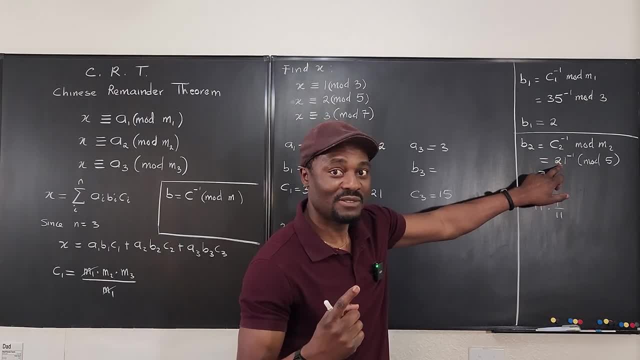 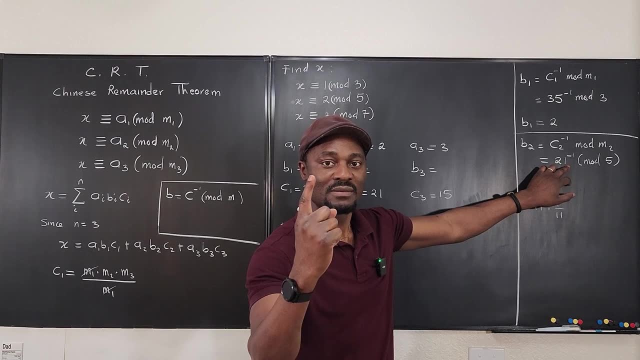 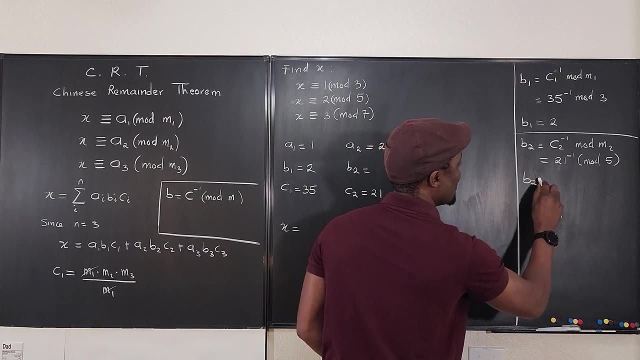 Just multiplying by 1, because 21 itself, divided by 5, leaves a remainder of 1.. So it means that the inverse of 21 mod 5 is 1.. That's the number that it has to be multiplied by. So we can say from here that b2 is equal to 1.. 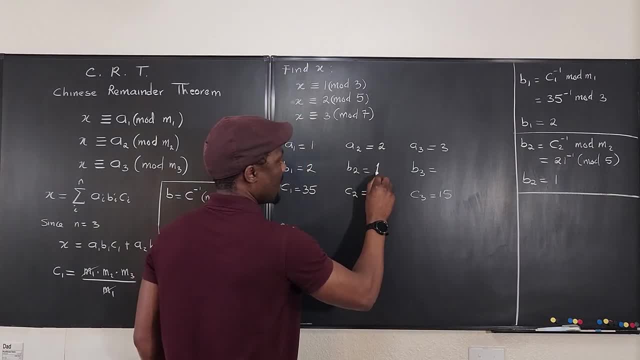 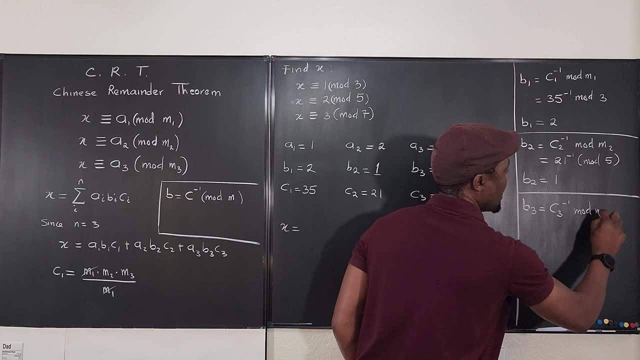 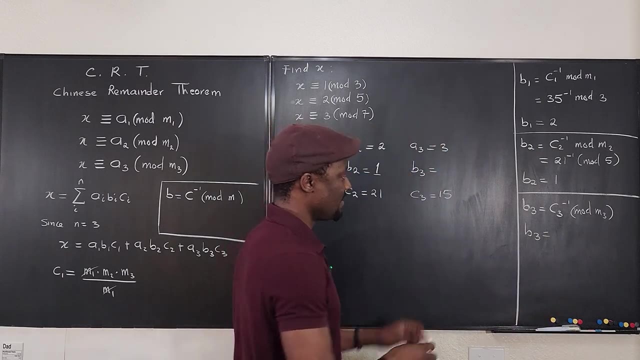 That's it. And then we go to the third one. So we say b3 is equal to c3, inverse mod m3.. Okay, So which means that b3 equals What is our c3? 15. The inverse of 15 mod 7.. 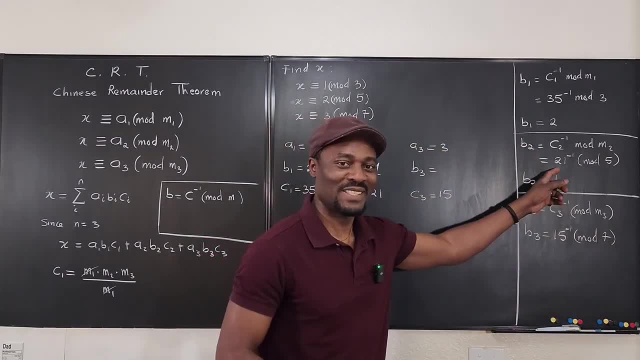 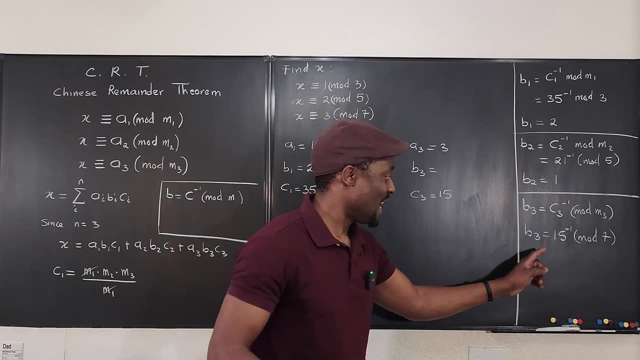 Okay. So the same thing, similar to this case, Just looking at 15.. If you divide 15 by 7, the remainder is 1.. That's it. So the inverse of 15 mod 7 is 1, because you only need to multiply 15 by 1. 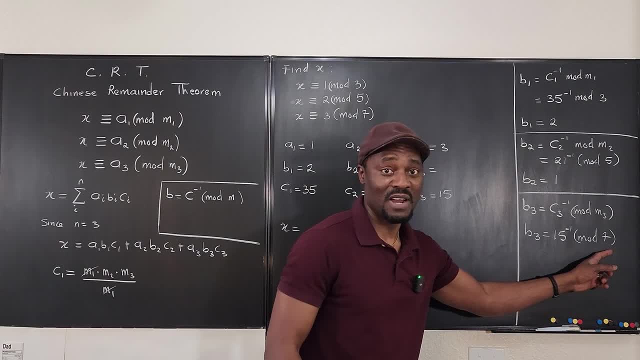 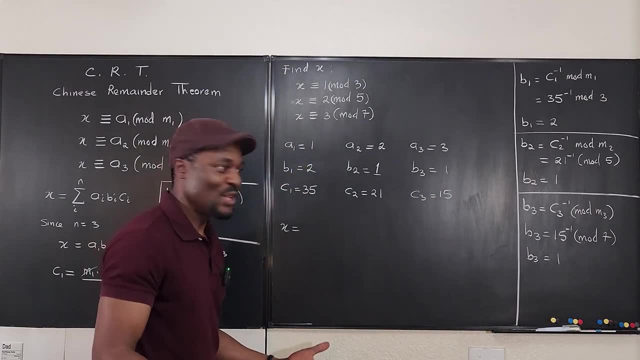 to get a situation where the remainder is going to be 1 when you divide by 7.. So we can say that b3 is equal to 1.. So we can fill this And we're done. So the number we're looking for. 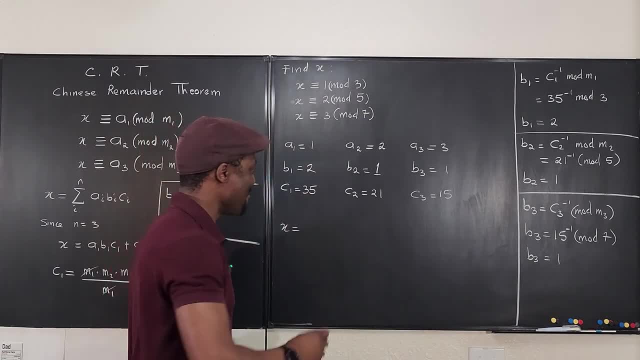 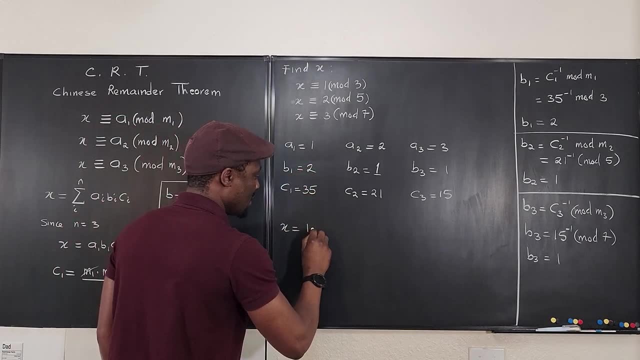 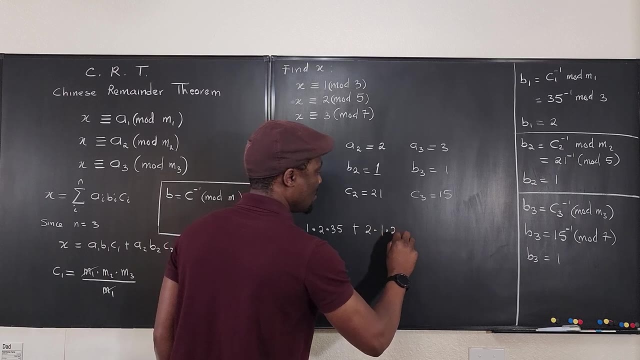 this mysterious number is going to be generated immediately, because we just have to multiply a1 by b1 by c1. And that gives us 1 times 2 times 35, plus 2 times 1 times 21, plus 3 times 1 times 15.. 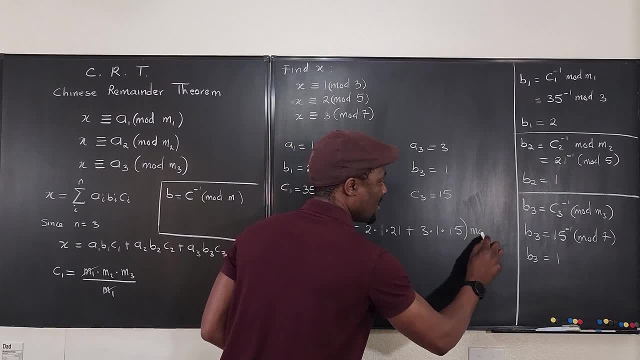 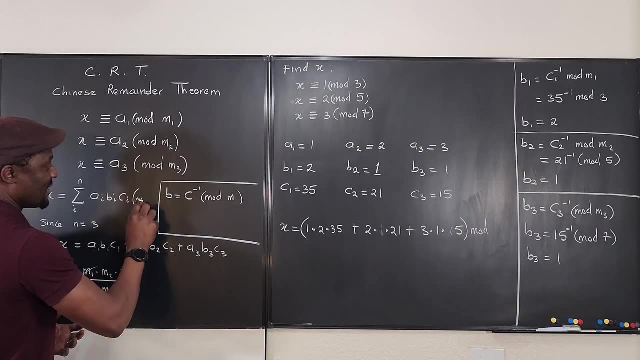 And all of this will be written mod giant m. Where is the giant m? Oh, I didn't write it. Oh, it's going to be mod giant m. Okay, And the giant m remember is is the product of the small m's. 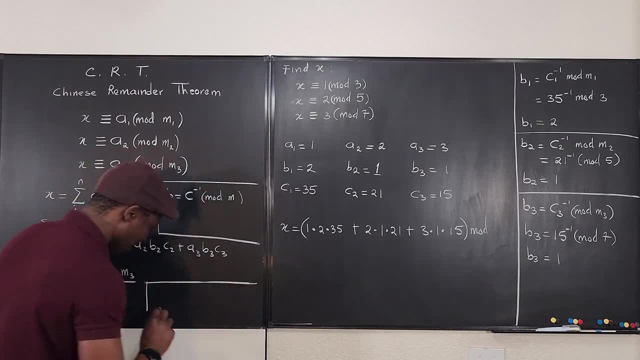 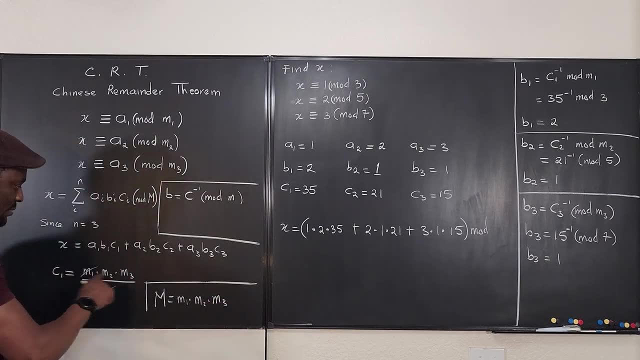 So remember that the giant m- Let's put that here- The giant m is equal to m1 times m2 times m3.. I think- Oh, I was supposed to write it here. So this is giant m, Okay. 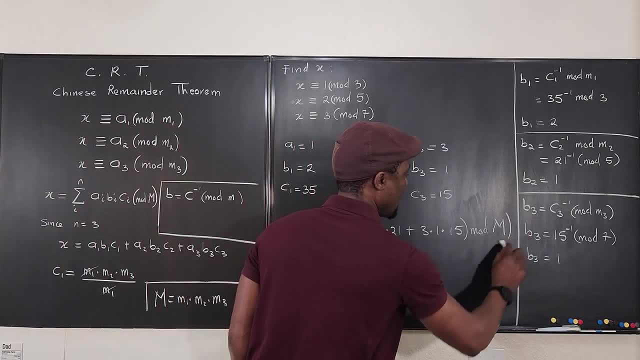 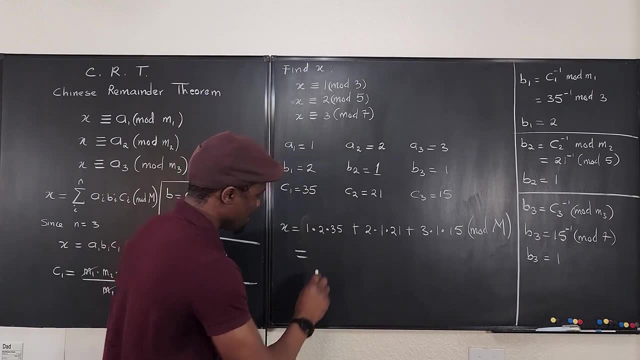 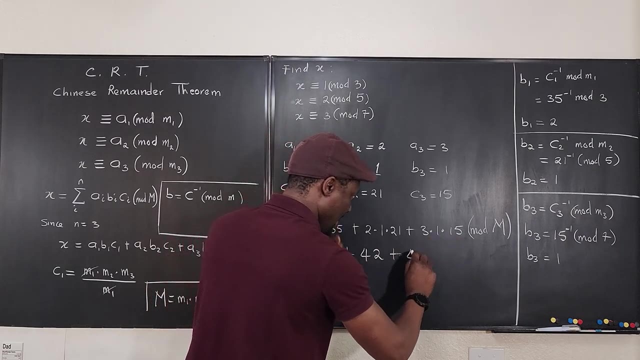 Now mod the giant m. Okay, We don't have to put this here, So that's what we have. So what do we have here? This is 70.. Plus 42. Plus What is this? 45.. 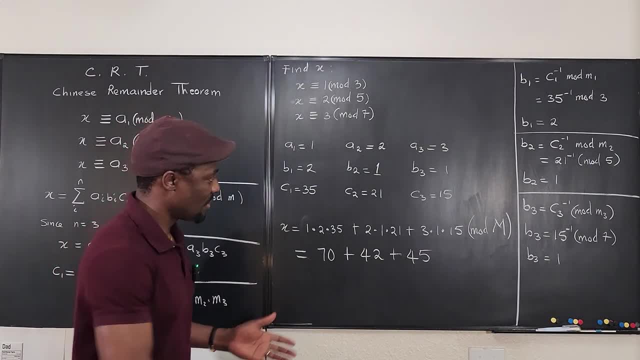 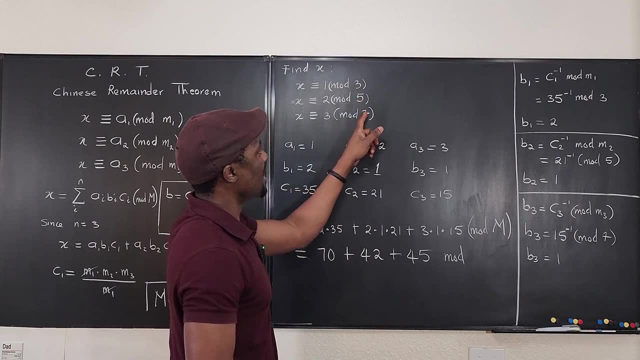 Okay, If we add, Let's use numbers, So it's going to be mod. What's the giant m? again, It's going to be 3 times 5 times 7.. That's 35 times 3.. 105.. 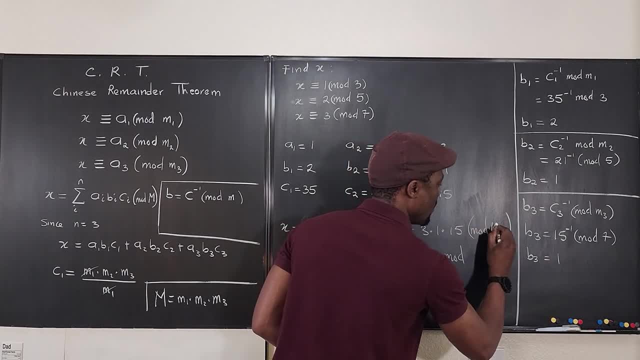 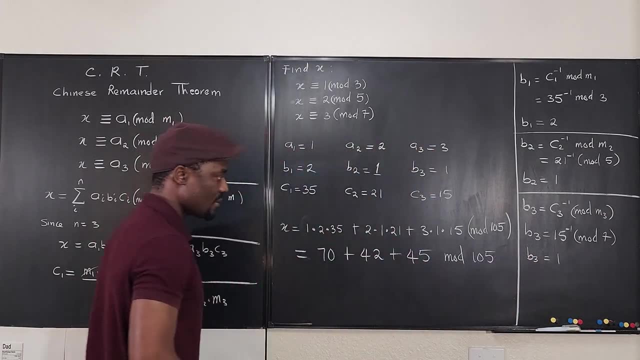 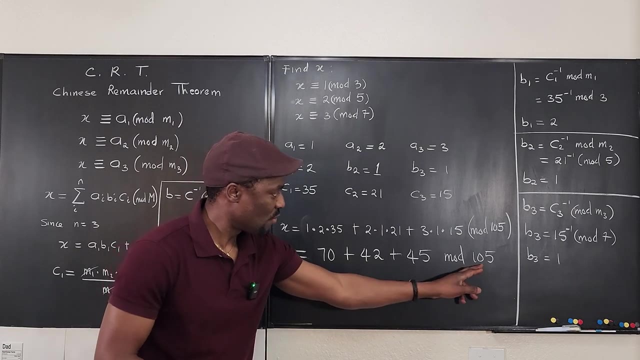 Let me write this as 105.. Because that's what we need: 105.. Okay, Nice, Mod, 105.. Let me write this, Okay. so How do you get the answer? Well, let me get as close to 105 as possible.